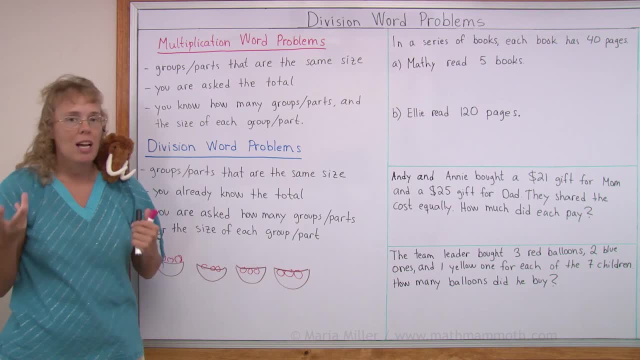 That, okay, I have so many apples. I have 24 apples, or 40 apples, or so many apples- And then I want to put them into baskets And either you have to solve how many baskets or how many apples goes into each basket. 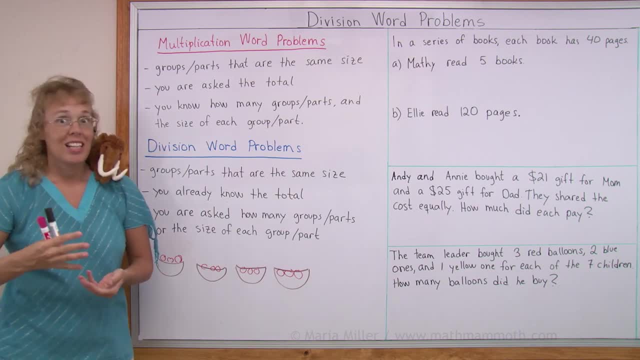 Okay. So I might tell you that, okay, there's 40 apples and 4 baskets. How many apples in each? Or I might tell you that there are 40 apples and I want to put 10 apples in each basket. 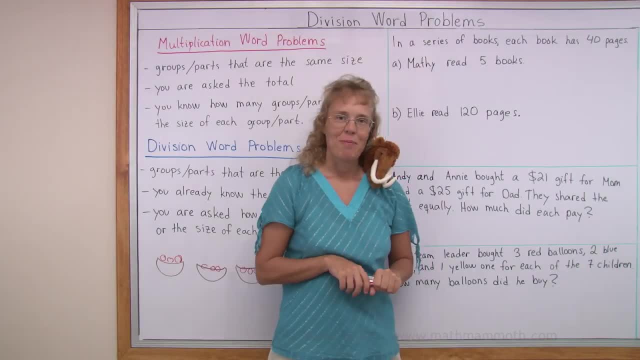 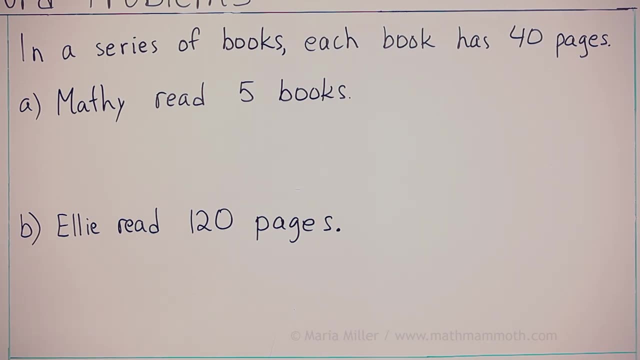 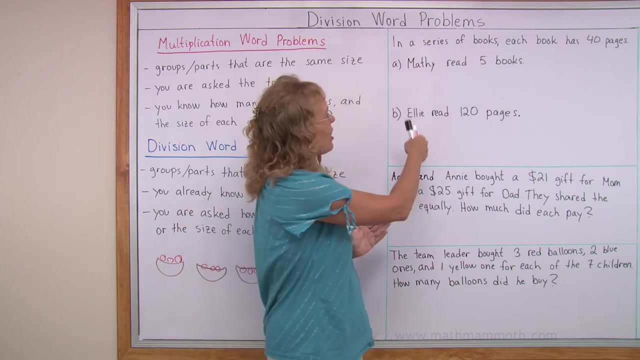 How many baskets? Okay, Okay, over here we have a situation: We have a series of books and each book has 40 pages. So here we have things that each have the same amount of pages, And now one of these will match a multiplication word problem. 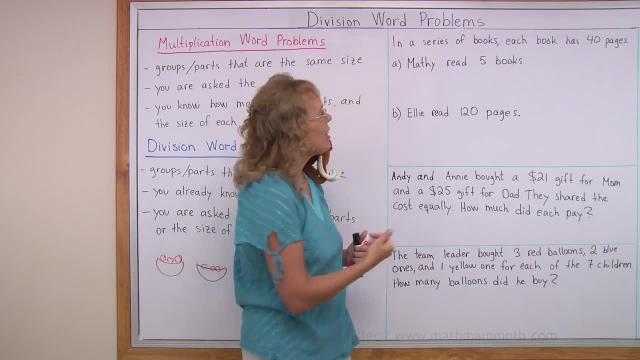 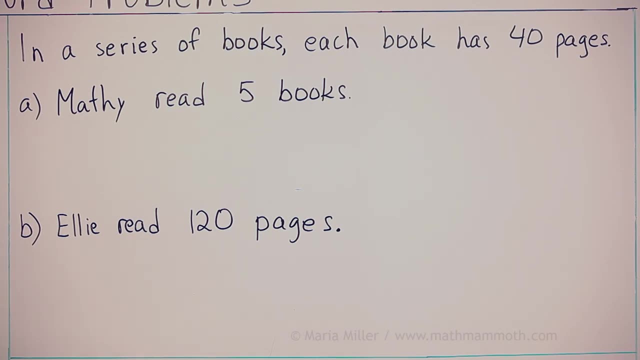 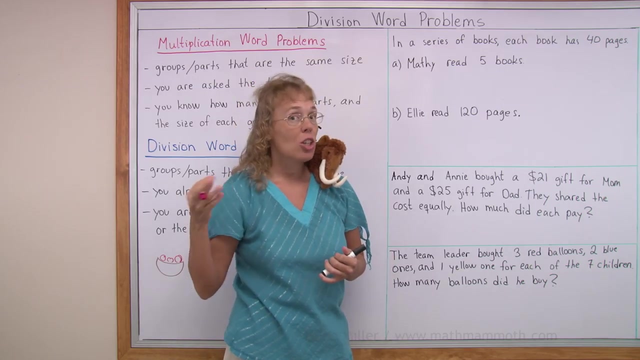 and one of them will match or be a division word problem. I didn't put the question here, so you can think about it. okay, Each book has 40 pages and Matthew read 5 books, So what could we ask? We could, of course, ask: how many pages did he read in total? 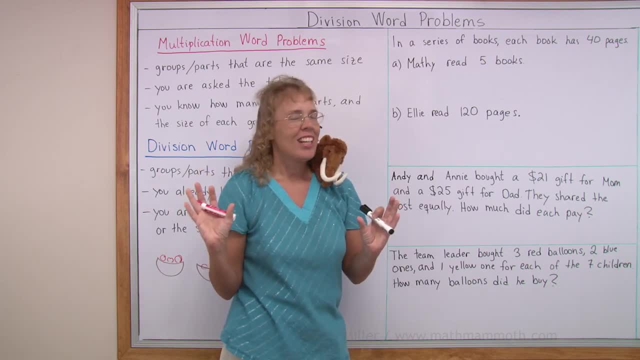 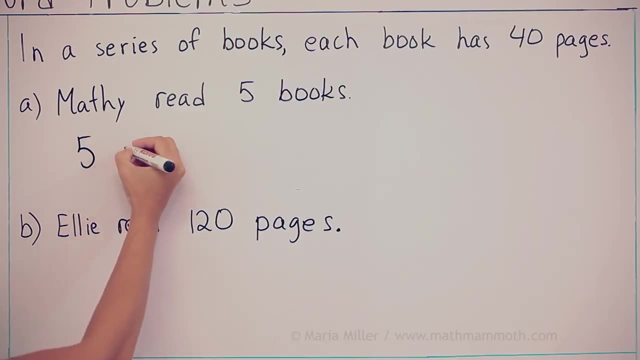 The total number of pages. Okay, And how would you solve it? You would write a multiplication right: 5 books times 40 pages In each book And you can add to find that 40,, 40,, 40,, 40,, 40.. 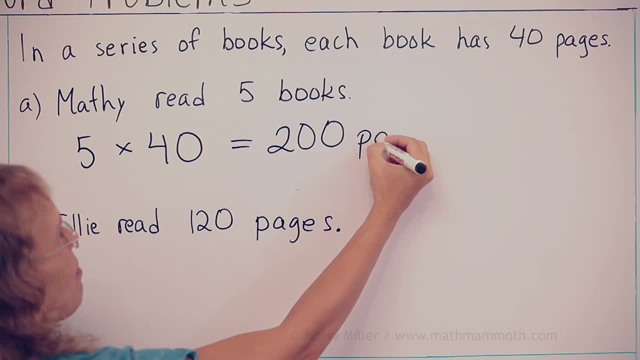 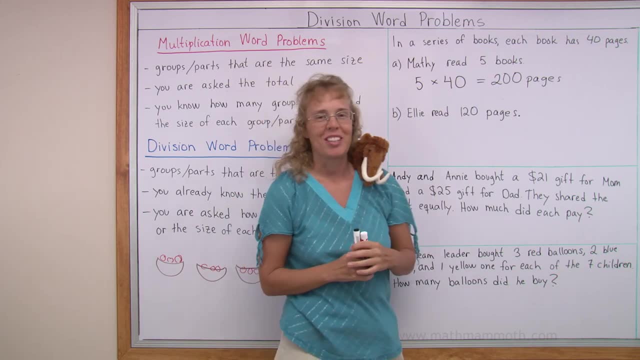 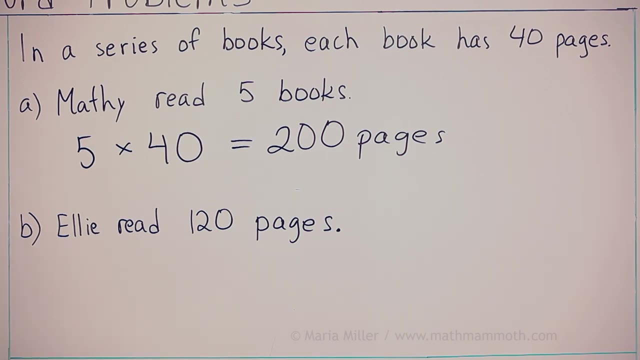 You should get 200 pages. So what kind of books were they? Matthew Math story books, Okay, I guess. so Here another. Ellie read 120 pages. She read those same kinds of books. What can we ask this time? 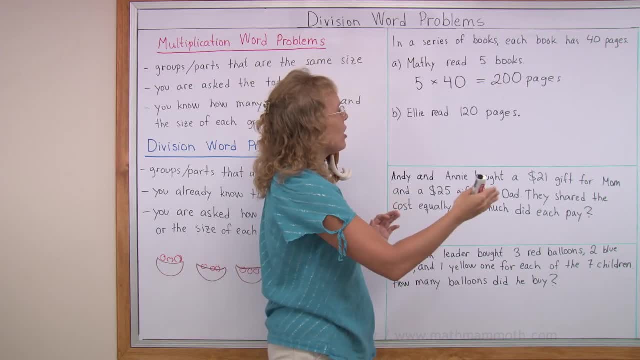 What can we solve? She read 120 pages. She read so many books, but we don't know how many. So we will ask: how many books did she read? And to answer that question can I write a multiplication or a division? 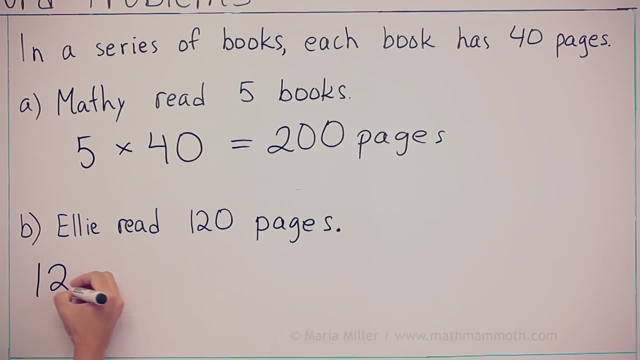 Okay, I can write a division: 120 divided by 40, right? And if those numbers look big to you, it's still an easy division. Just think this way: How many 40s are in 120?? The answer is 3, right. 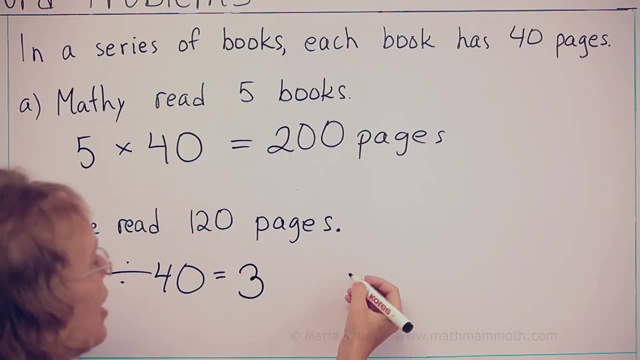 I can also write a multiplication this way. In this multiplication I would not know how many books there are, So I leave that empty. It's my unknown. And then times 40 pages equals 120 pages. I know the total, okay. 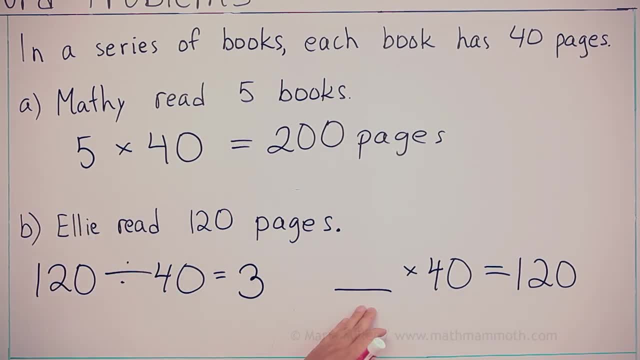 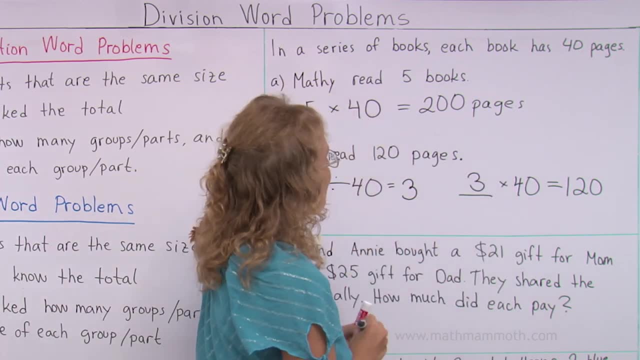 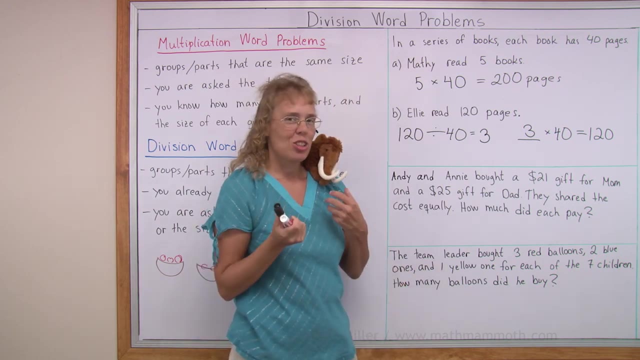 And so I would write the total here, And then 3 goes here. This would be a missing factor problem. One of the numbers, The number we multiply, is missing. And now, lastly, I have two problems for you to solve that are actually mixed. 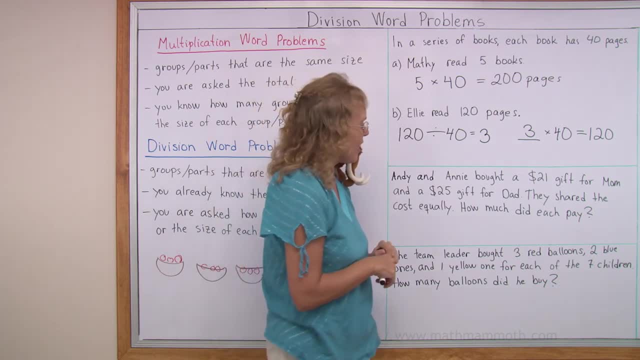 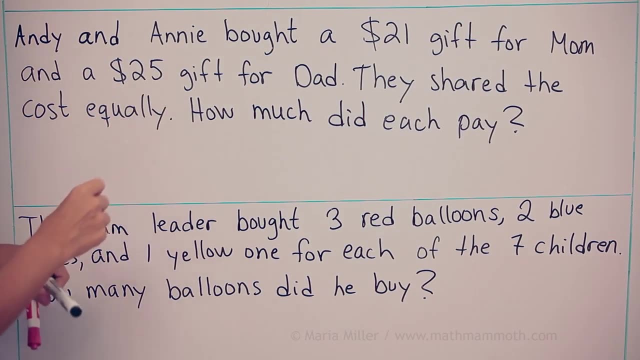 They require several operations. okay, So they are not just simple multiplication or division problems. Andy and Annie bought a $21 gift for mom and a $25 gift for dad. They shared the cost equally. How much did each pay? All right, they buy two things. 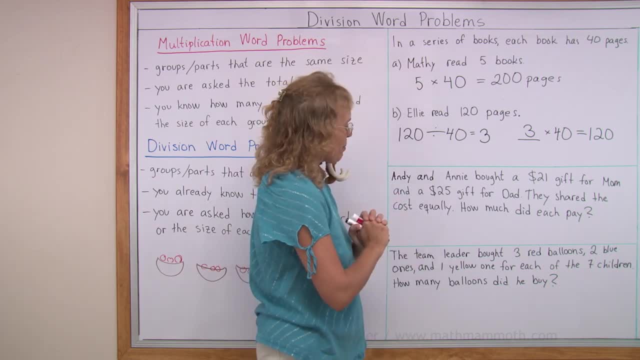 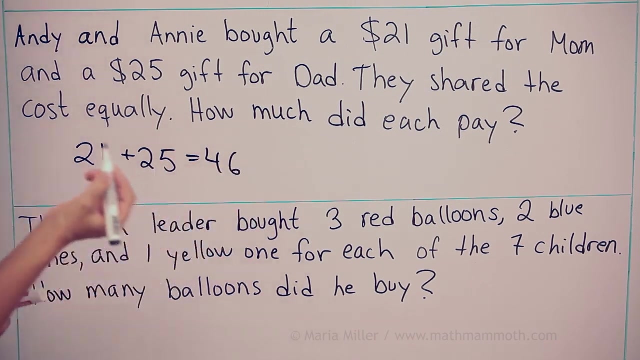 They share the cost. So what would you do? They buy two things. Let's first find how much those two things cost together just by adding. Okay, there's 21 plus 25.. That's 46.. It's $46.. 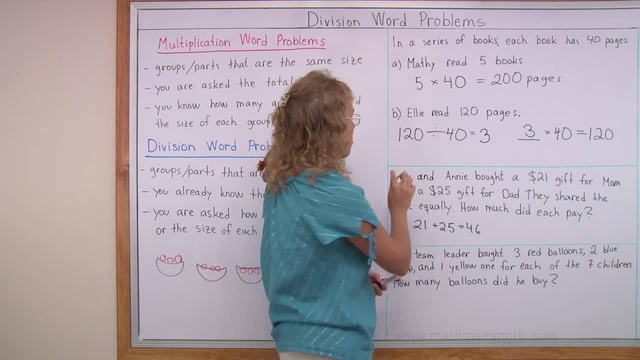 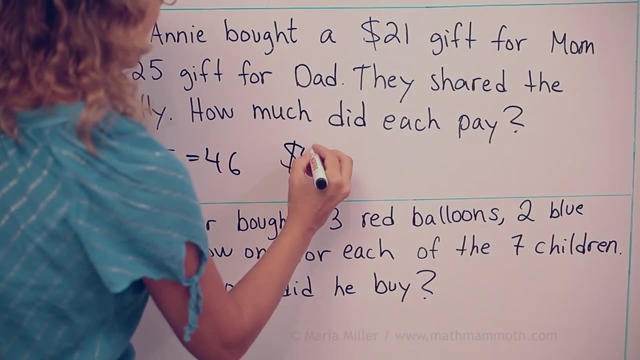 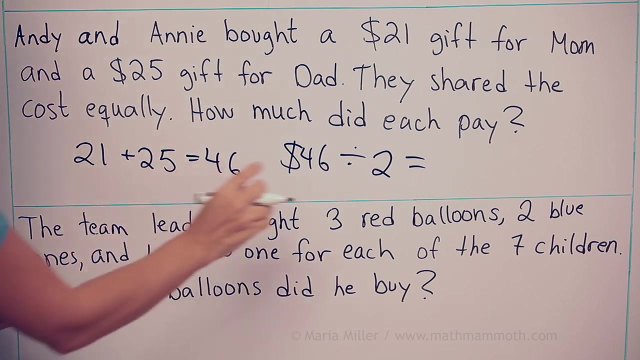 And then they share the cost equally in those two people. Maybe it's a brother and sister And We would divide right. Let me write here $46 and divide by two, And how much will each pay? Take half of this number. 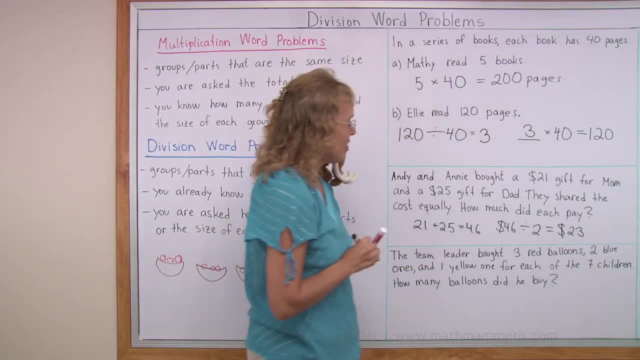 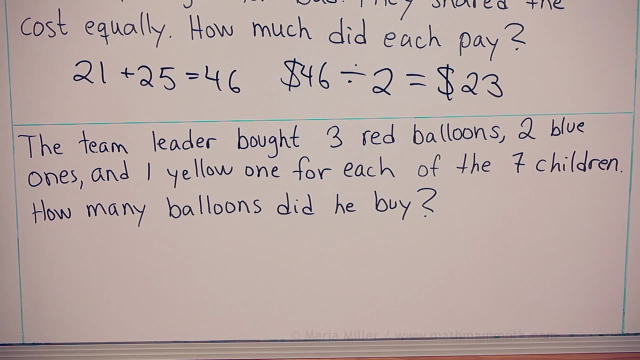 Simply $23.. Okay, so that one took two operations and this one will too. The team leader bought three red balloons, two blue ones and one yellow one for each of the seven children. So how many balloons did he buy? How many balloons in total did he buy? 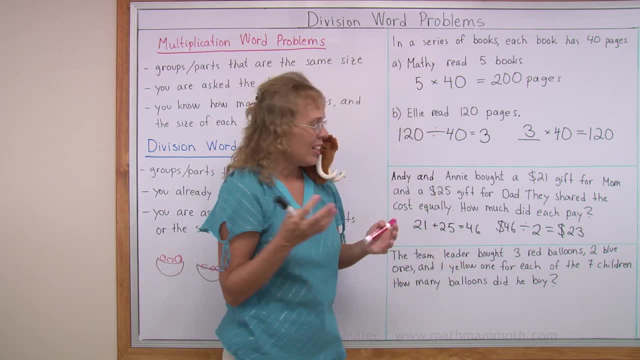 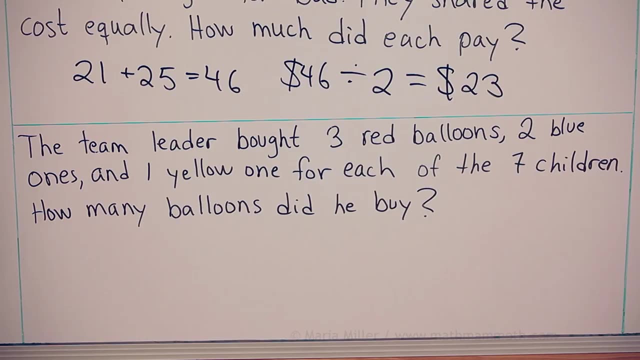 How many balloons in total did he buy? Okay, since we don't know the total, it might have to do with multiplication, right? Okay, since we don't know the total, it might have to do with multiplication, right. Those three red balloons, two blue ones and one yellow, one for each child. 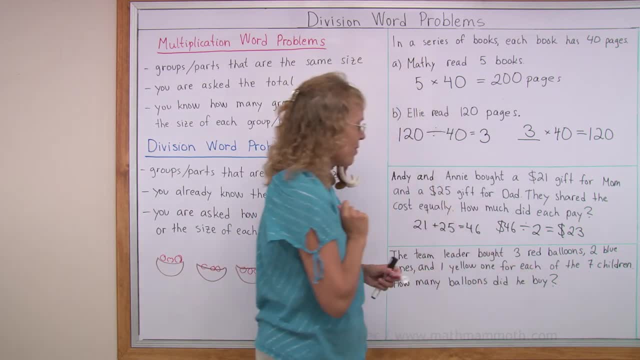 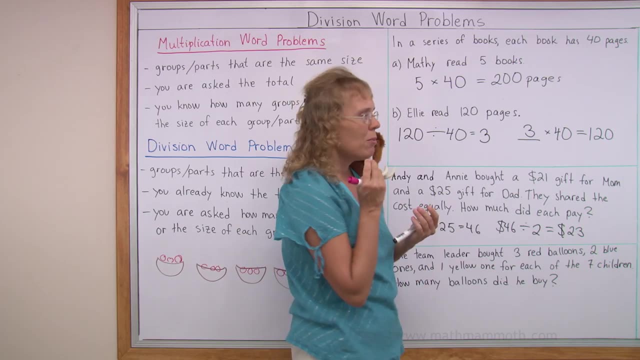 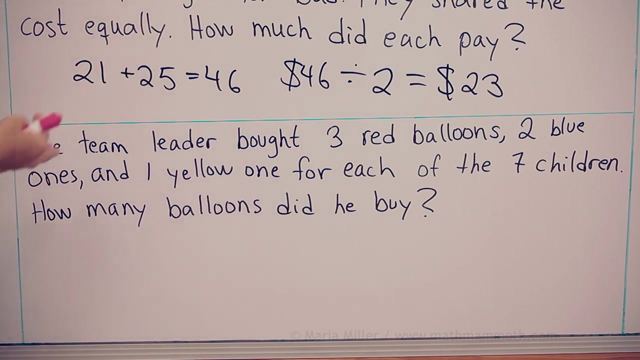 Another clue word is this: each. Okay, when there is the each, it might be multiplication or division. Seven children Now, how many balloons does each child get? Six balloons, right, You have to add three plus two plus one. Six balloons for each child.